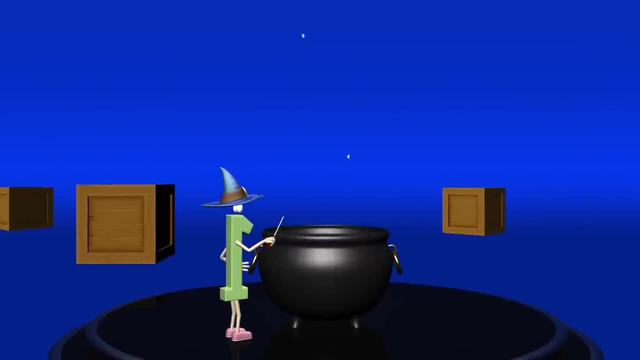 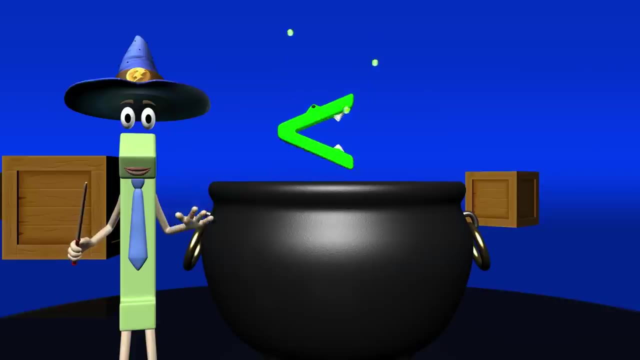 Abra-ka-bibble: No, that's not it. Alaka-fraction: No, not that either. Oh, hey guys, I am practicing some magic to try and make something appear out of this pot. This is the magical fraction. 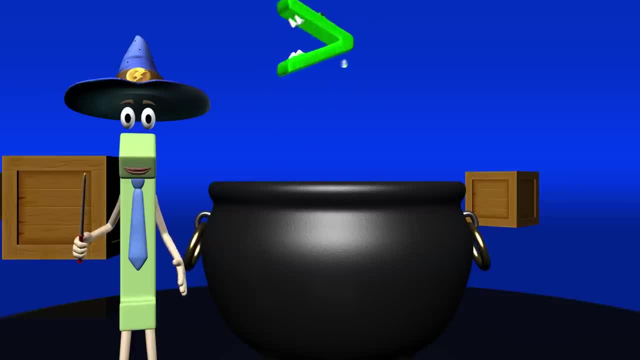 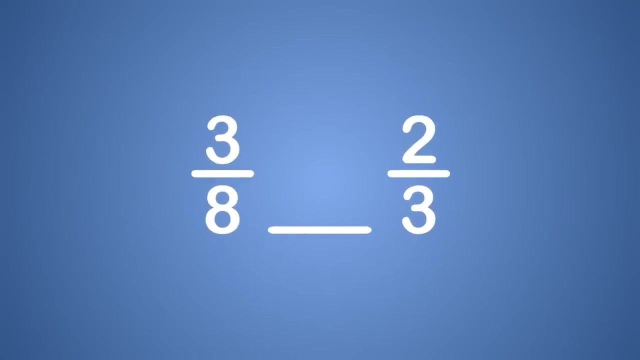 pot. I use this pot to compare fractions and supposedly it can be used for magic spells to make things appear, but so far nothing. Let's learn together about comparing fractions and maybe I will get the spells right. Here are two fractions. Which fraction is greater? 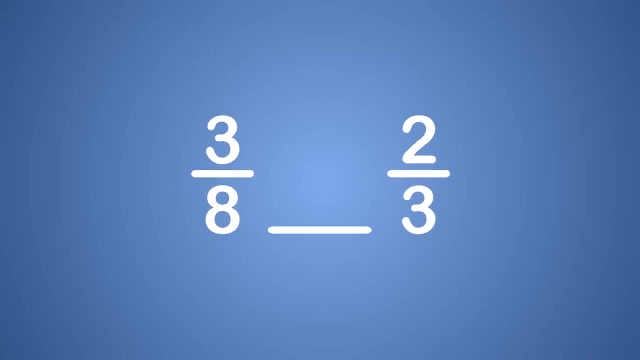 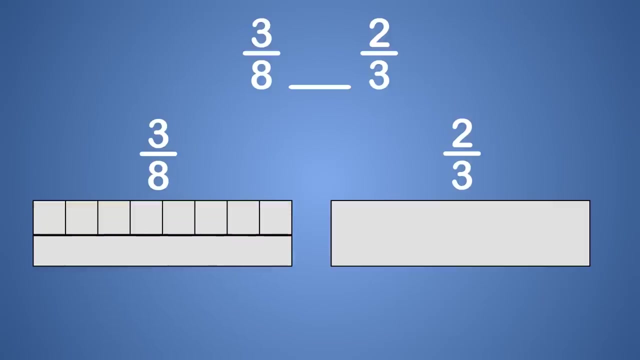 three-eighths or two-thirds. Let's compare the fractions with models. Start by drawing two rectangles that are the same size. Then we partition the rectangles to show the fractions. The rectangle on the left gets divided into eight equal parts. Now we need to shade three. 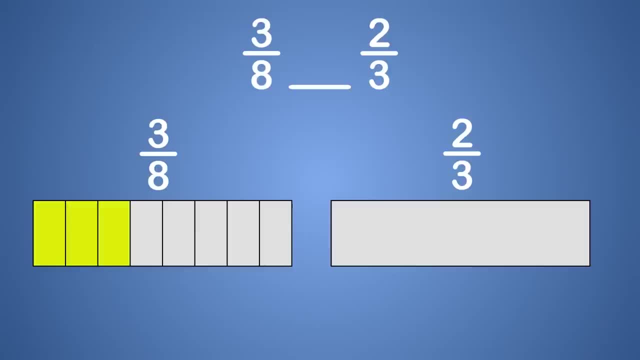 parts to make the fraction three-eighths. This represents three-eighths. Now we look at the rectangle on the right Partition, the fraction on the right into three equal parts. Now we shade two parts. This represents two-thirds. Notice, the length of shaded region in the fraction on the right is longer than the shaded 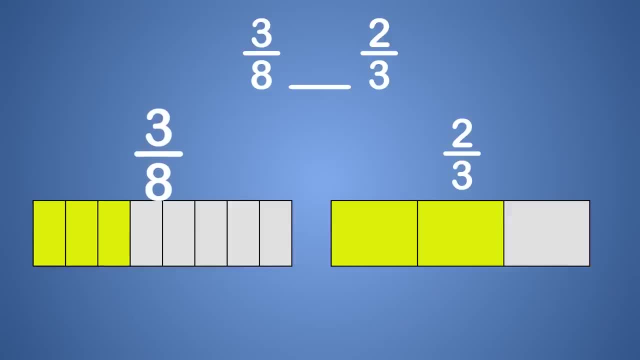 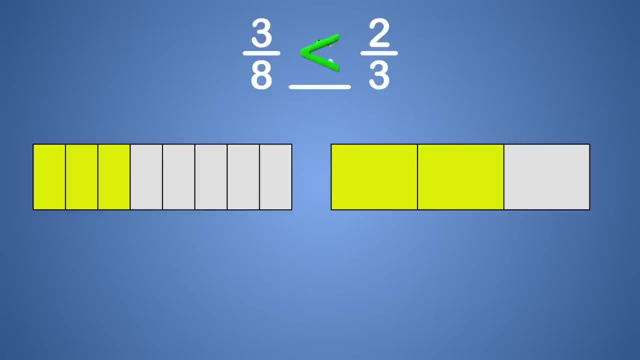 region in the fraction on the left. That means three-eighths is less than two-thirds. We will write a less than symbol in the blank. So the problem reads: three-eighths is less than two-thirds. Just in case you forget which direction the symbol faces: always have the open part towards. 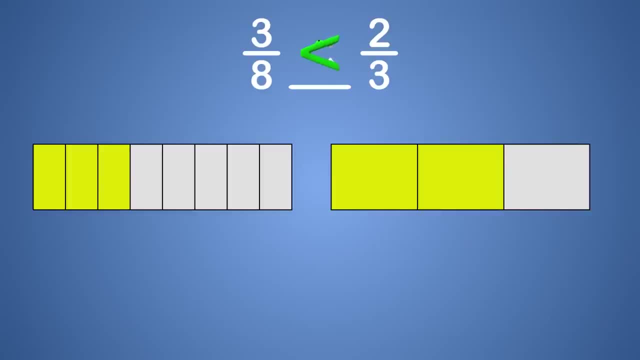 the larger number. Think of it as a hungry, hungry alligator that likes to eat large numbers. Let's try another problem: Which fraction is greater, four-eighths or three-sixths This time? let's try a different method. Let's write both fractions with a common denominator. 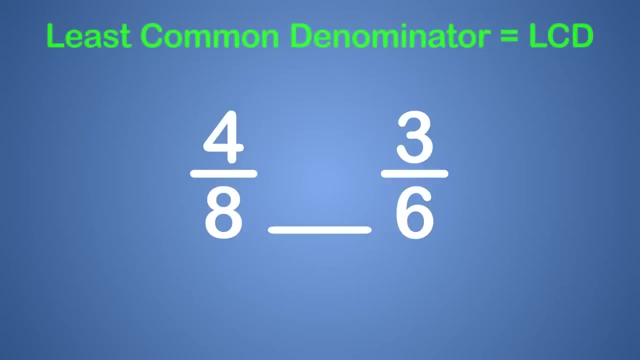 First we need to determine the least common denominator, or LCD. The LCD is the lowest possible multiple of the two denominators. Our denominators are eight and six. Next let's list a few of their multiples. Eight times one is eight. 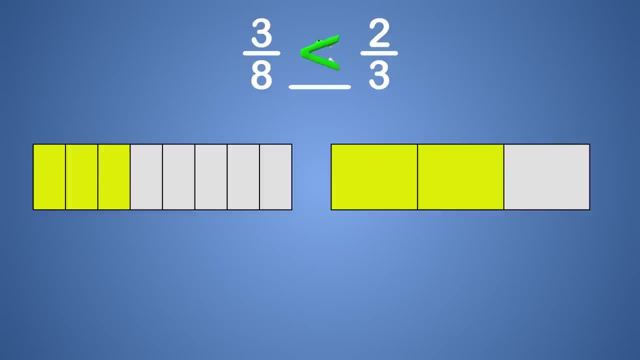 the larger number. Think of it as a hungry, hungry alligator that likes to eat large numbers. Let's try another problem: Which fraction is greater, four-eighths or three-sixths This time? let's try a different method. Let's write both fractions with a common denominator. 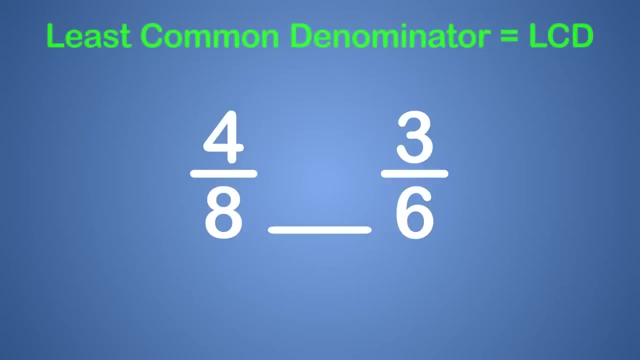 First we need to determine the least common denominator, or LCD. The LCD is the lowest possible multiple of the two denominators. Our denominators are eight and six. Next let's list a few of their multiples. Eight times one is eight. 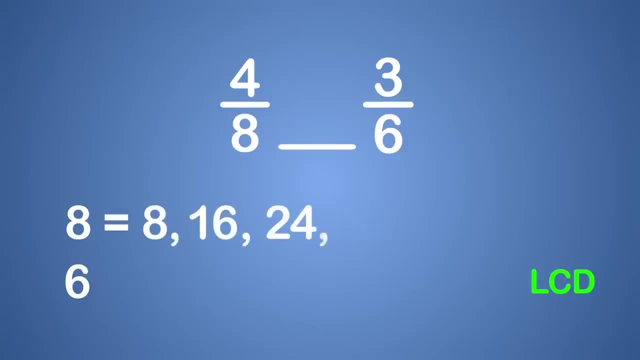 Eight times two is sixteen. Eight times three is twenty-four. Eight times four is thirty-two, And so on. Okay now, six, Six times one is six. Six times two is twelve. Six times three is eighteen. Six times four is twenty-four. 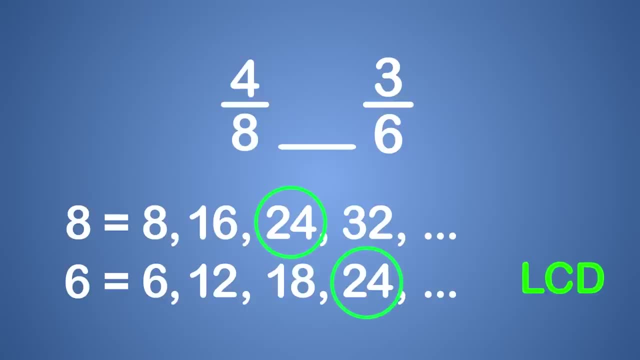 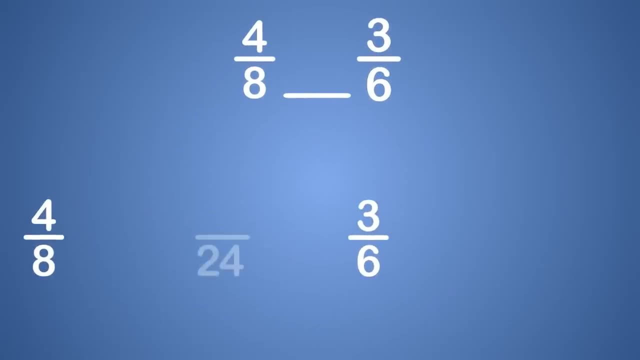 And so on. Aha, Twenty-four is the lowest common multiple of eight and six. This will be the new denominator in our fractions. Now let's write four-eighths as a fraction with twenty-four in the denominator. What number times eight is twenty-four? 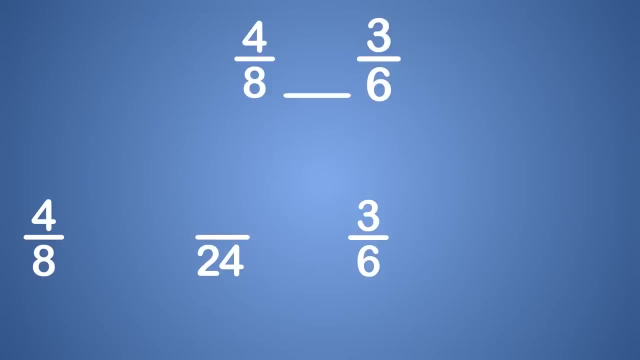 That's right, three. So we will multiply both the numerator and denominator by three to get an equivalent fraction. Four times three is twelve and eight times three is twenty-four. We found four-eighths is equivalent to twelve twenty-fourths. 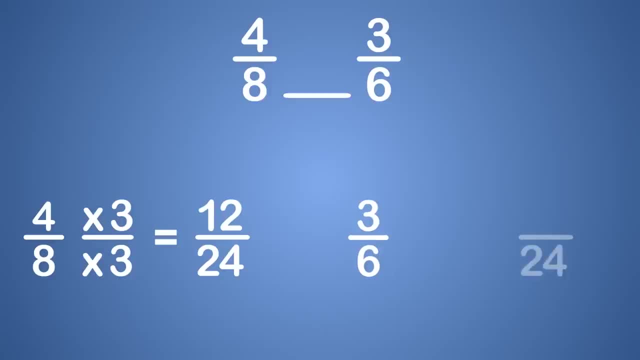 Now let's write three-six as an equivalent fraction with a denominator of twenty-four. What number times six is twenty-four, That's right, four. So we will multiply both the numerator and denominator by four to get an equivalent fraction. Three times four is twelve. 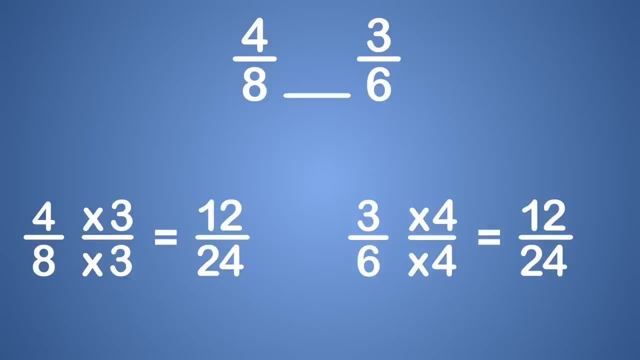 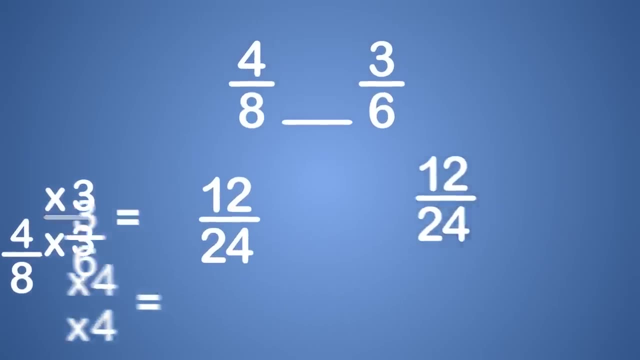 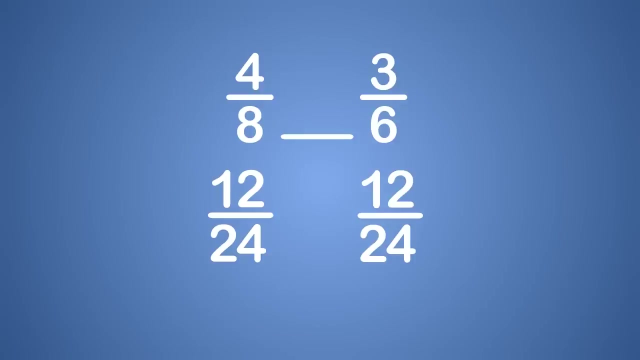 And six times four is twenty-four. We found that three-sixths is equivalent to twelve twenty-fourths. So let's compare the equivalent fractions. Which symbol do we use? Greater than, less than or equal to Twelve twenty-fourths and twelve twenty-fourths are equal to each other. 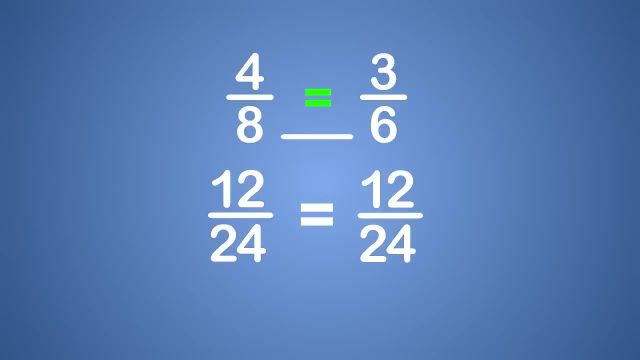 Awesome job. We compared the fractions by making an equivalent fraction. So four-eighths is equal to three-sixths- Sweet. Let's look at another problem. Let's compare these two fractions, four-sixths and two-thirds. Which one is larger? 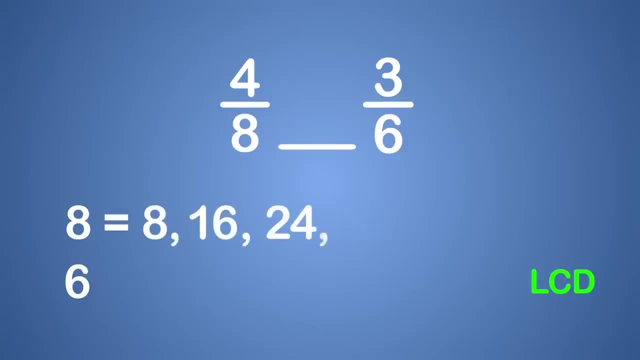 Eight times two is sixteen. Eight times three is twenty-four. Eight times four is thirty-two, And so on. Okay now, six, Six times one is six. Six times two is twelve. Six times three is eighteen. Six times four is twenty-four. 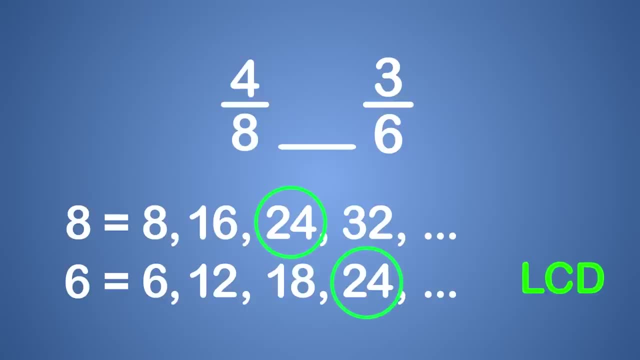 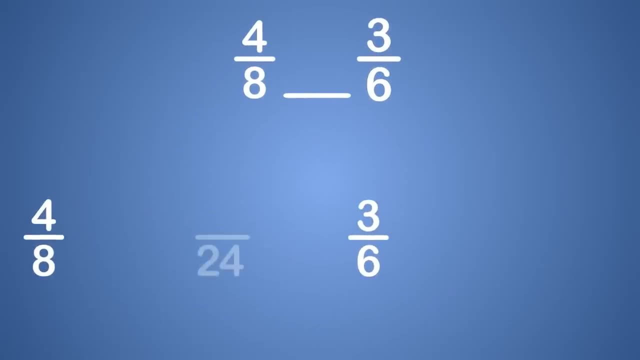 And so on. Aha, Twenty-four is the lowest common multiple of eight and six. This will be the new denominator in our fractions. Now let's write four-eighths as a fraction with twenty-four in the denominator. What number times eight is twenty-four? 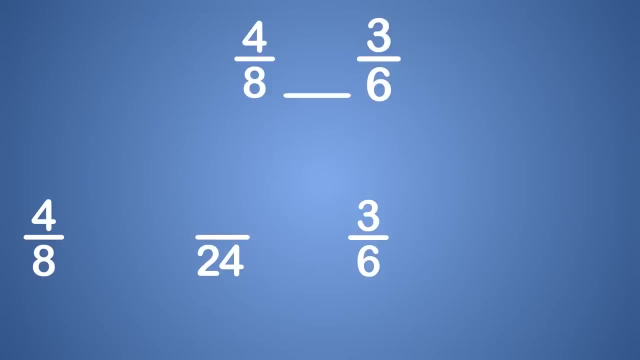 That's right, three. So we will multiply both the numerator and denominator by three to get an equivalent fraction. Four times three is twelve and eight times three is twenty-four. We found four-eighths is equivalent to twelve twenty-fourths. 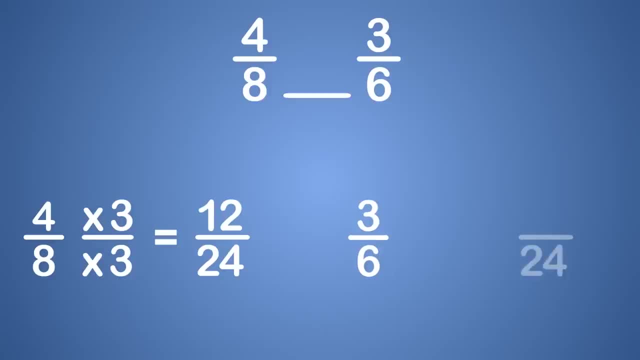 Now let's write three-six as an equivalent fraction with a denominator of twenty-four. What number times six is twenty-four, That's right, four. So we will multiply both the numerator and denominator by four to get an equivalent fraction. Three times four is twelve. 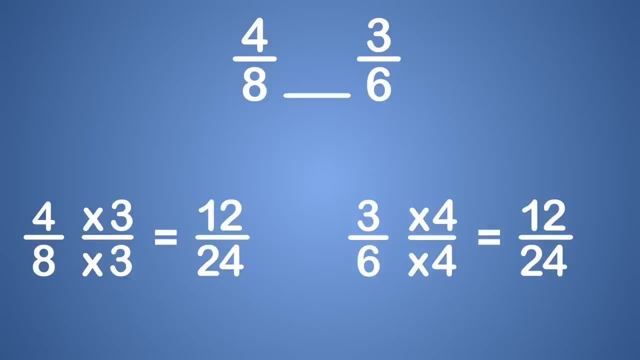 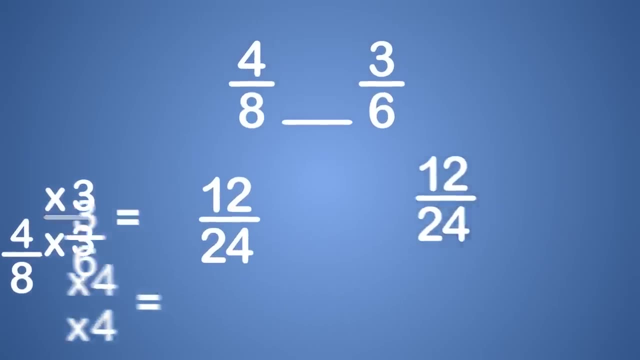 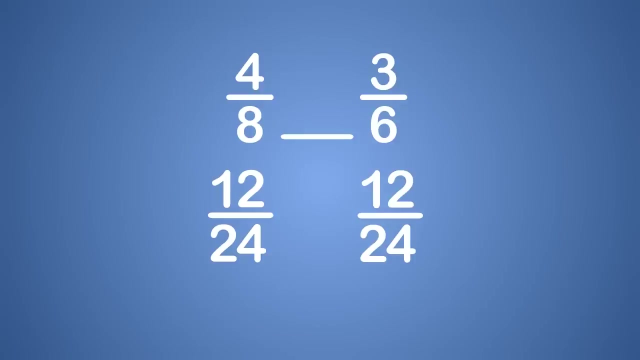 And six times four is twenty-four. We found that three-sixths is equivalent to twelve twenty-fourths. So let's compare the equivalent fractions. Which symbol do we use? Greater than, less than or equal to Twelve twenty-fourths and twelve twenty-fourths are equal to each other. 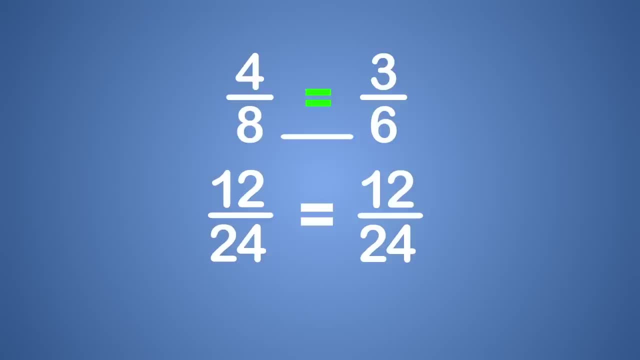 Awesome job. We compared the fractions by making an equivalent fraction. So four-eighths is equal to three-sixths- Sweet. Let's look at another problem. Let's compare these two fractions, four-sixths and two-thirds. Which one is larger? 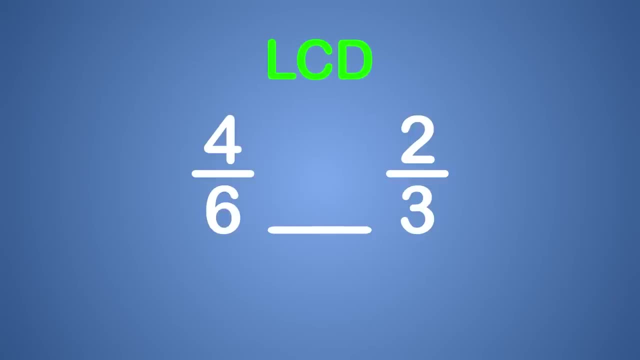 Let's start by finding the LCD or least common denominator for six and three, by listing some of their multiples. Some multiples of six are six, twelve, eighteen and so on. Some multiples of three are three, six, nine and so on. 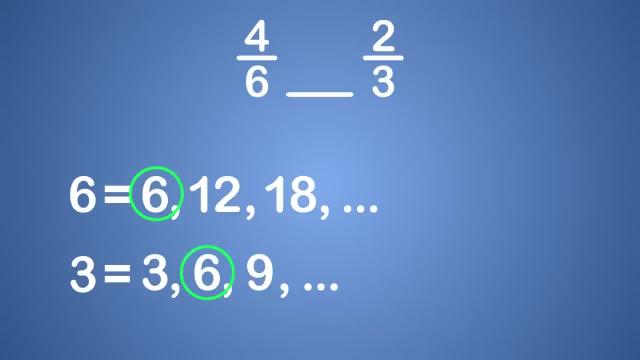 The least common multiple of six and three is six. Now we know the least common denominator to use. But waitfour-sixths already has a denominator of six. Sweet, We don't have to touch this fraction, so let's change two-thirds into an equivalent fraction.